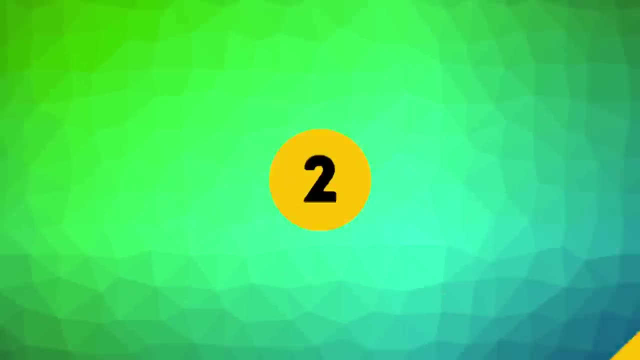 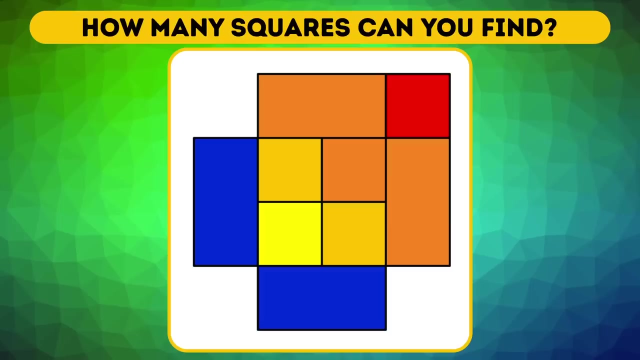 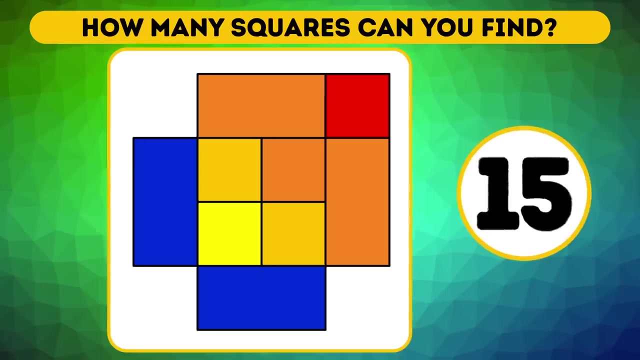 Number eight, Number seven, And now you got 30!. Number nine, Number 20.. Number 20.. Okay, already. Number дв Two, Number one: You already tried 50 times perfect. You saw so much difference you gained. 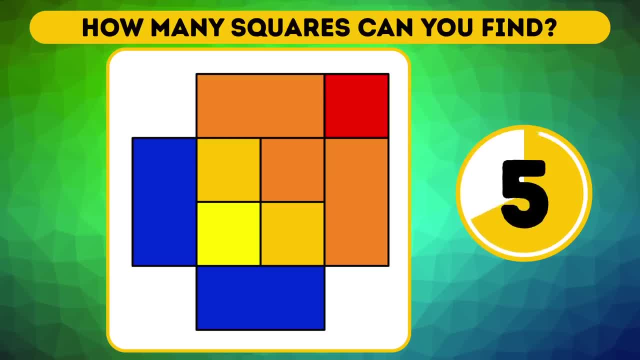 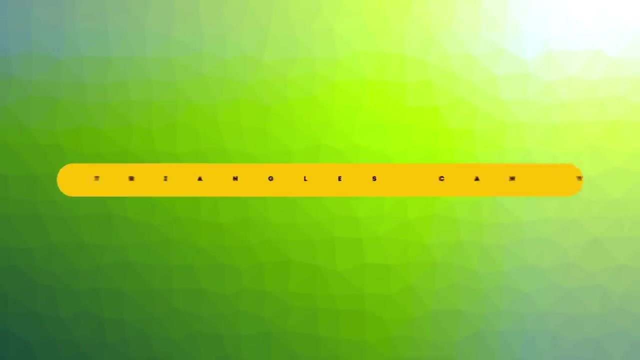 You nailed it. Number five. Numbers nine: up time's ticking away. There are 11 squares in this image. Here's how you can find them. Number three: Alright, let's take a break from staring at squares and give this pentagon a try. 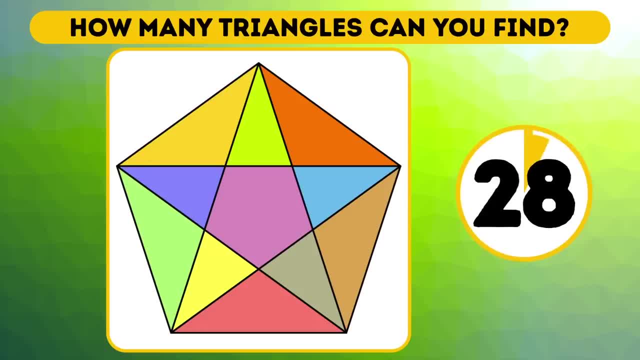 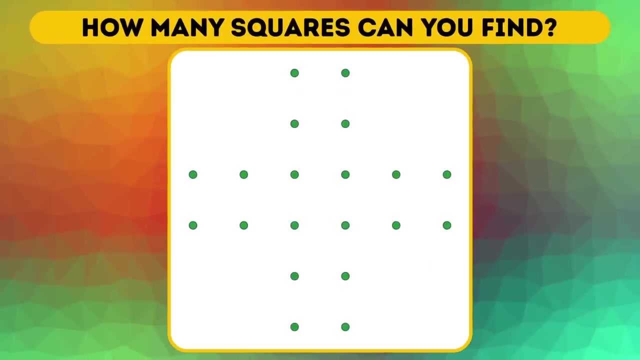 How many triangles does it have? Take your time, this one's tough. You've got 10 more seconds And the answer is: drumroll. please. 35 triangles in a variety of shapes, In a variety of sizes. Number four: This cross is hiding something from you, And that something is perfect squares. 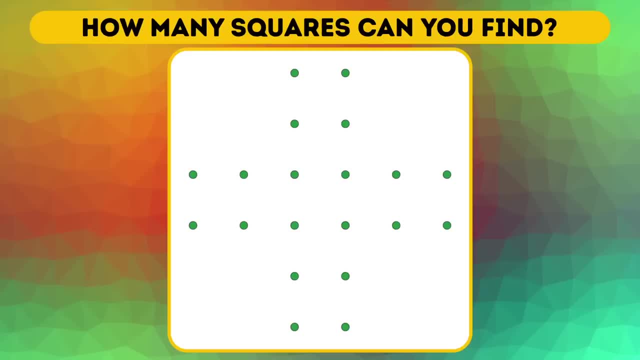 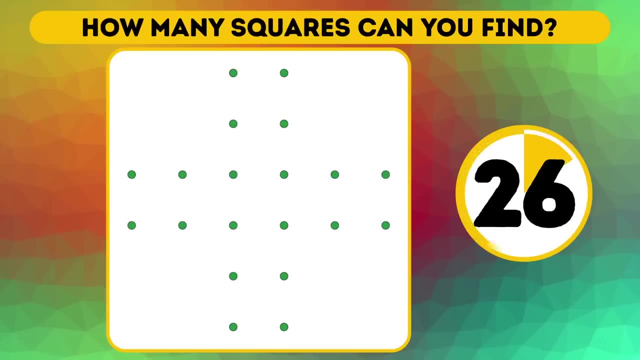 They consist of four dots, with one on each corner. So how many are there? You've got half a minute, so get to counting Number five. The correct answer is 21 squares. That's even more than the number of dots in the cross. 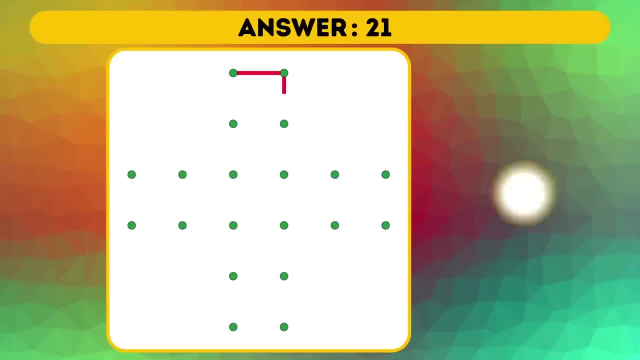 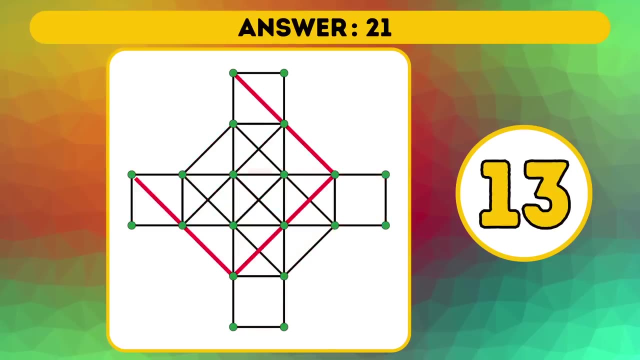 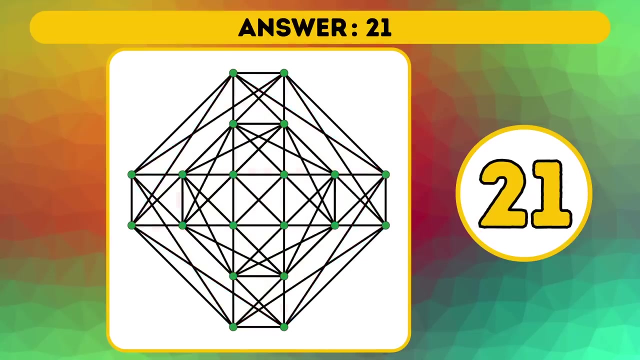 Wanna know how to find them. Check it out. Number five: How many triangles does it have? You've got half a minute, so get to counting And that something is perfect squares. It's even more than the number of dots in the cross. 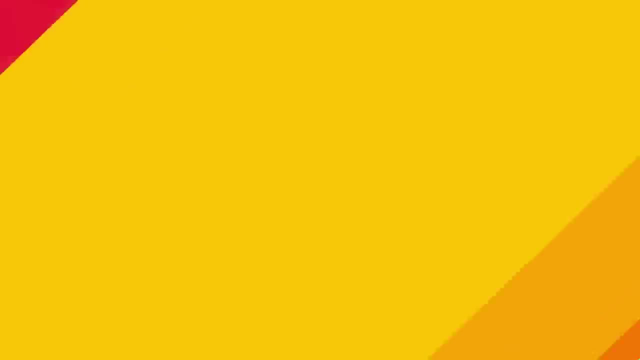 Wanna know how to find them. Check it out. Number five: How many triangles does it have? You've got half a minute, so get to counting. You've got half a minute, so get to counting. How many triangles can you find in this picture? 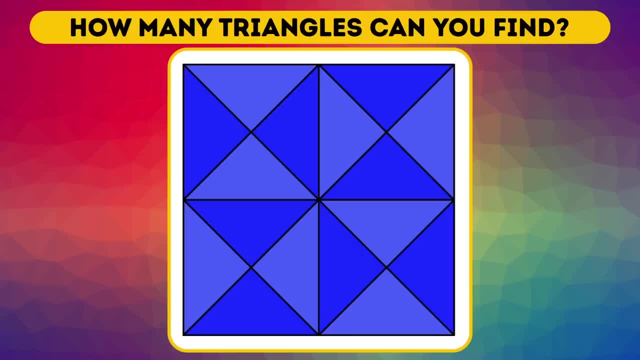 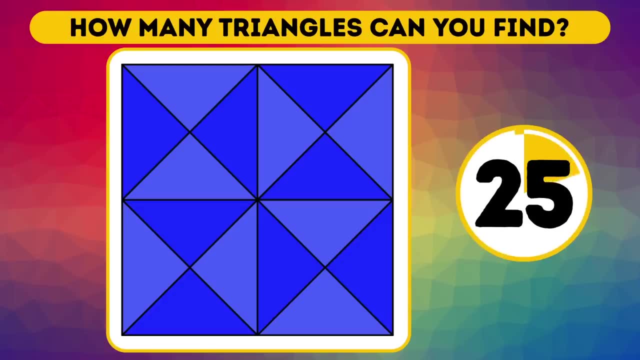 Remember all possible sizes and color combinations. count Your 30 seconds. start now llamas sonora. Did you spot 44?? In that case, good for you. If you couldn't find them all, here's a map to help you out. 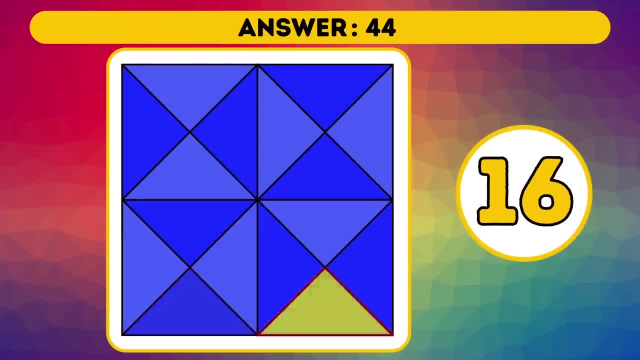 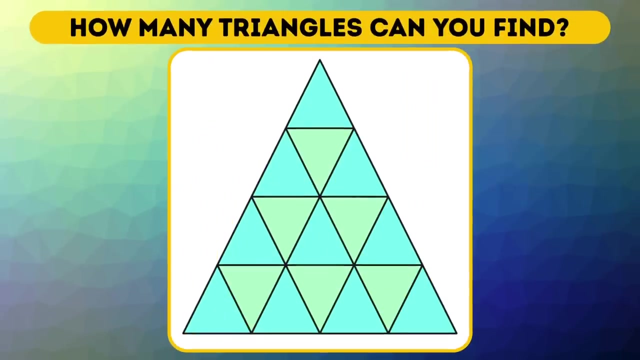 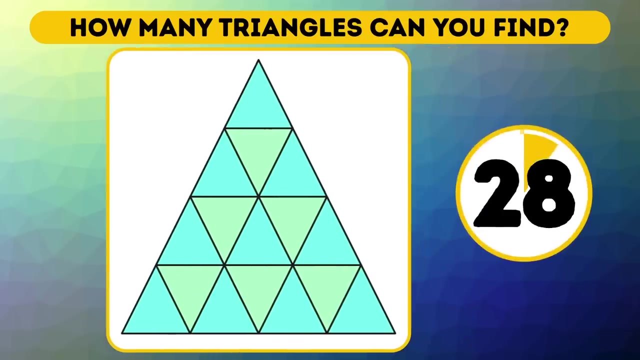 llamas sonora, number six. now we have one massive triangle. can you tell how many triangles, big and small, fit in here? you know the drill: 30 seconds on the clock. the answer is 27. want to hear the explanation? this formula will help you count the figures in any similar riddle. we have four triangles at the bottom of 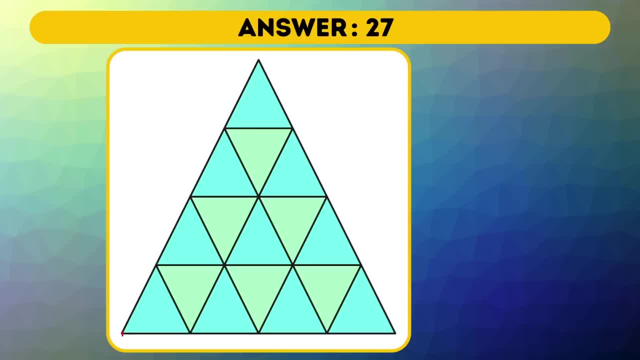 the big one. so let's start by counting how many triangles, big and small, fit in here. you know the drill: 30 seconds on the clock. many triangles have a side length equal to four. we've got one such triangle here and it's facing upward. now we can count the up facing triangles with three at. 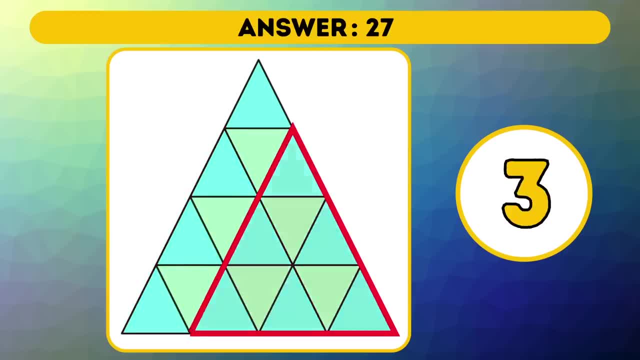 the bottom and we have three of them: two on the bottom row and one up higher. we continue like that, counting the triangles with size two and one. this way we can figure out there are twenty triangles facing up in this picture, for down facing triangles will count from the opposite direction. 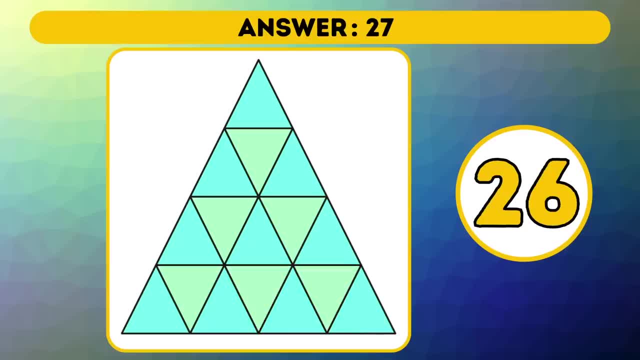 starting with size one. there are six of them here and just one triangle of size two facing down. it's the largest here. so after all this counting, we end up with 27 triangles in this picture number seven. after that last one, your brain could probably use a break. 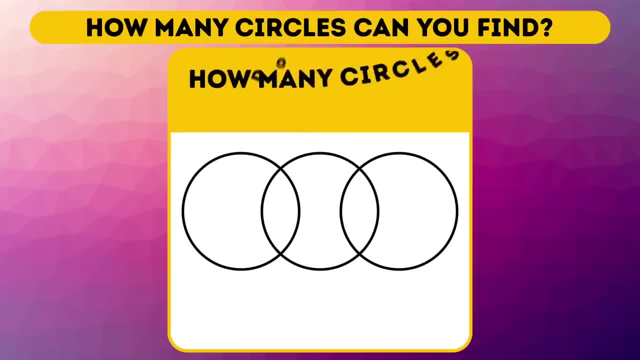 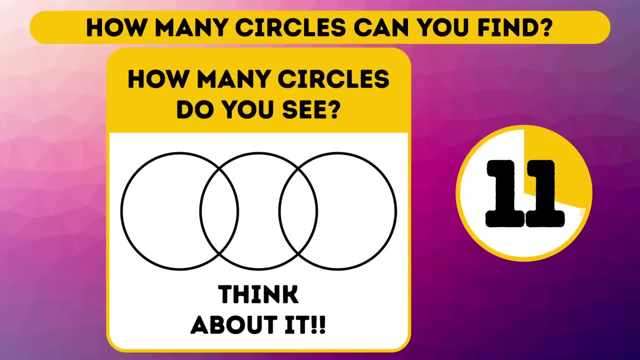 so how about an easy one? how many circles do you see here? three, Duh. Is that your final answer? I'll still give you 15 seconds to think it over. What if it's not that simple? after all, The correct answer is 10.. 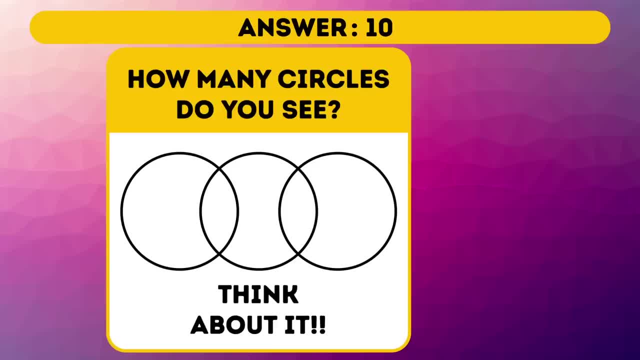 When I asked you to look for circles, I was talking about the whole image text included. There are four O's in the question, In how do you? and about No, we're not cheating. Then there's a question mark and an exclamation mark, both of which have round dots in them. 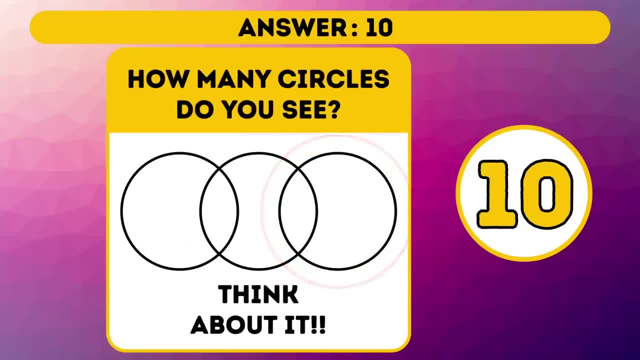 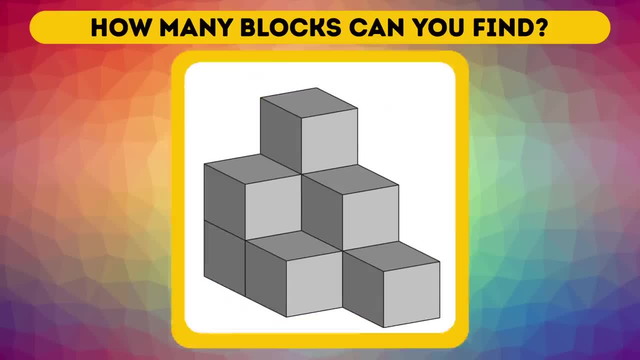 Add the three obvious circles and you get 10.. Alright, let's move on. before you start throwing things, Number 8.. Let's step things up with this 3D picture. You've got 15 seconds to decide how many blocks are in this picture. 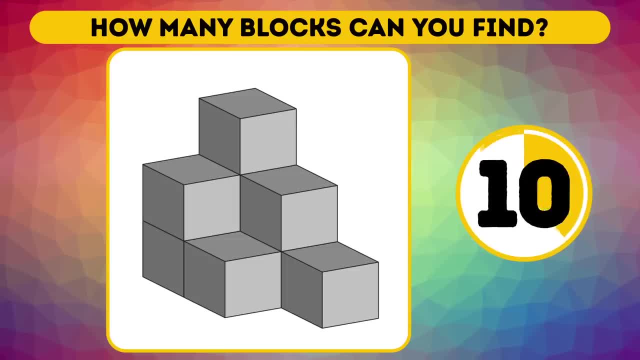 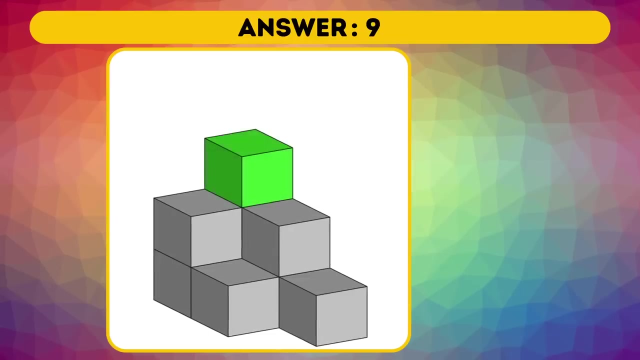 Time's up, The answer is 9.. The secret here is that there are some blocks that we can obviously see, but there are some hidden ones below the visible blocks. There's just one block on the top row. As for middle row, it has two blocks that we can see. 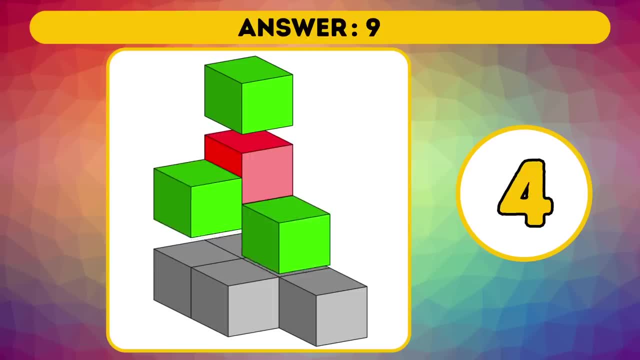 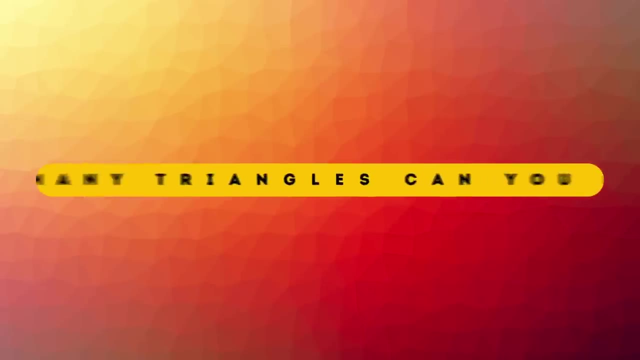 and one that we can't see, And it's hidden. supporting the top one. The bottom row has two hidden blocks and three obvious ones, And that's how we get nine blocks, Ta-da Number 9.. This one goes out to all you cat lovers.